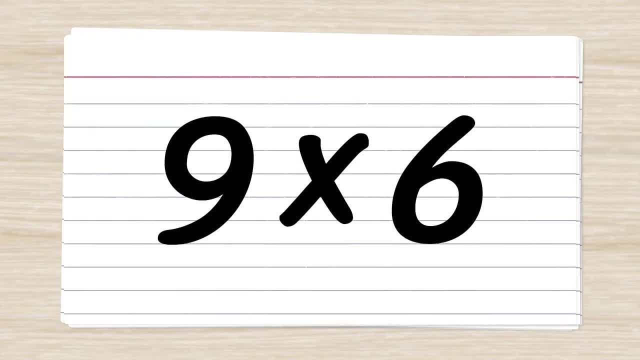 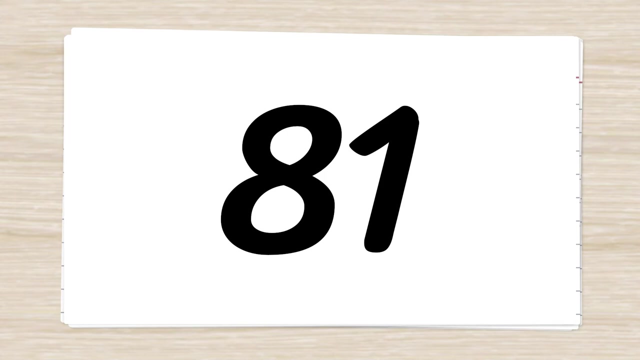 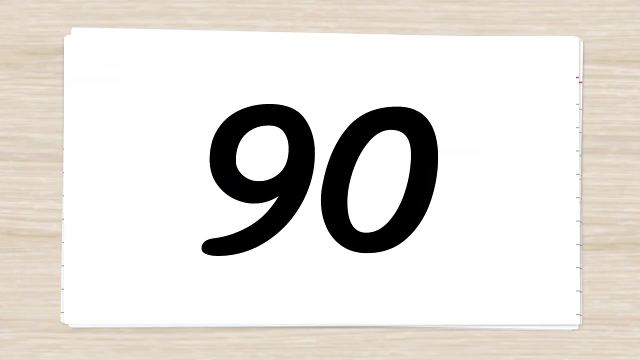 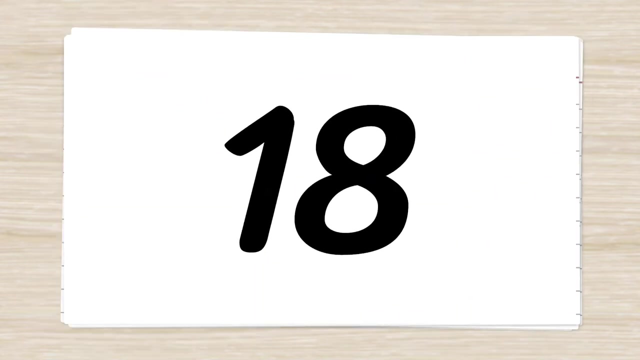 9 times 6.. 54. 9 times 7.. 63. 9 times 8.. 72. 9 times 9.. 81. 9 times 10.. 90. 9 times 2. 18.. 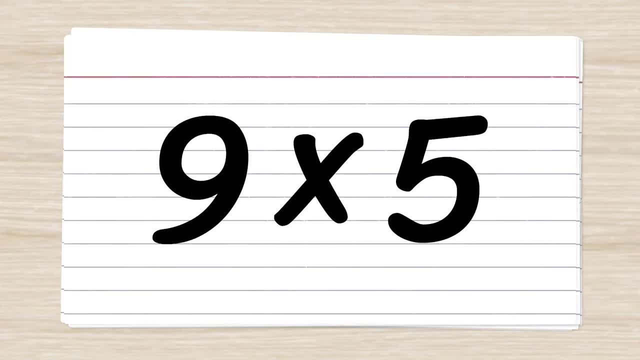 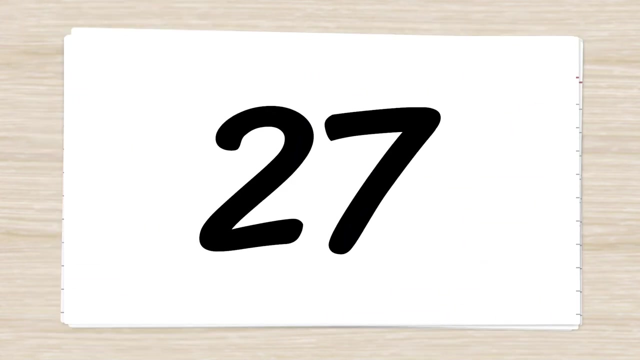 9 times 5.. 45. 9 times 7.. 45.. 63. 9 times 3.. 27. 9 times 6.. 54. 9 times 9.. 81. 9 times 1.. 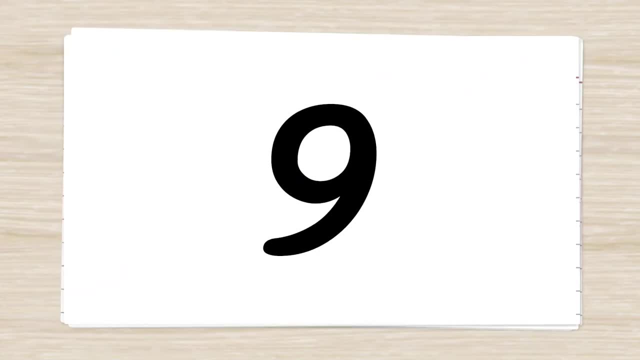 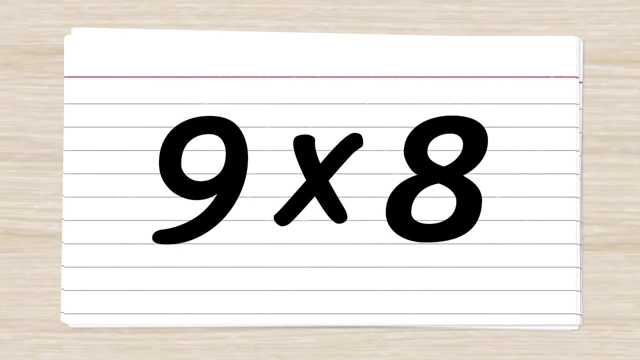 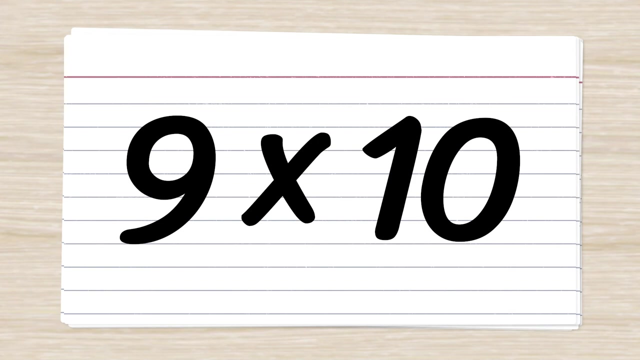 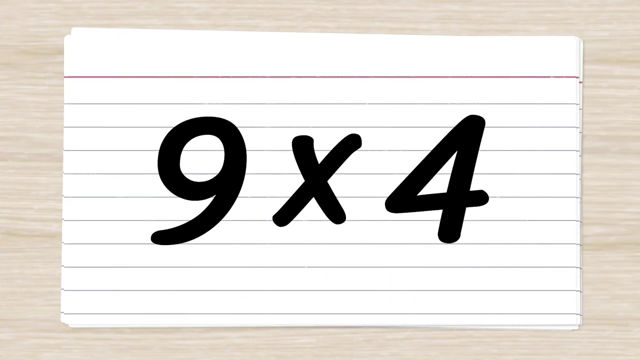 2., 2., 7., 7., 9., 9., 9., 7., 3., 3., 7., 7., 3., 9., 8., H, H. Thirty-six, nine, times zero, zero.